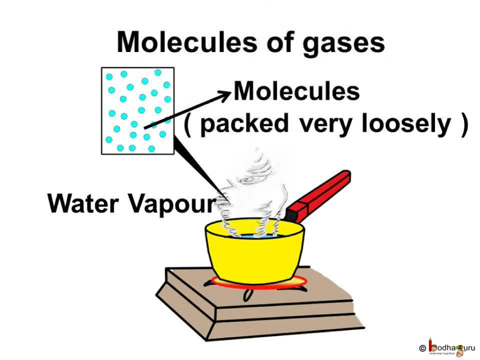 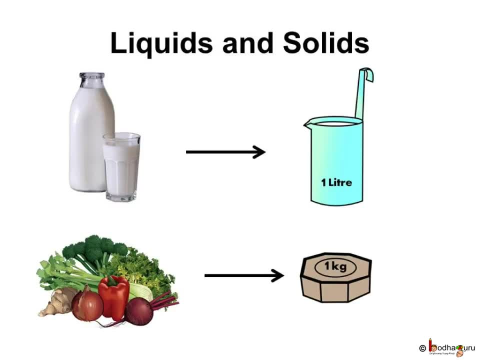 Gases do not have shape, but they have weight, although gases weigh much lesser than solids and liquids. We can measure solids and liquids, But the methods are different. When we buy milk it is measured in litres. It means we buy it by measuring how much space it occupies. 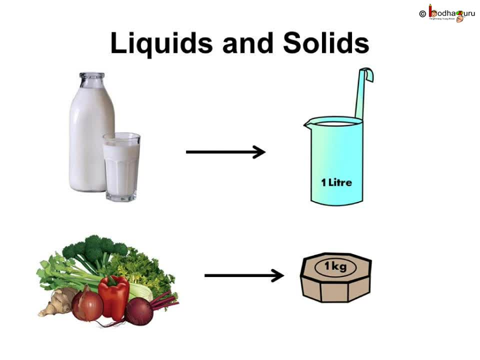 The amount of space occupied by an object is called its volume, And when we buy vegetables or sweets, it is measured by the volume. And when we buy vegetables or sweets, it is measured by the volume. And when we buy vegetables or sweets. 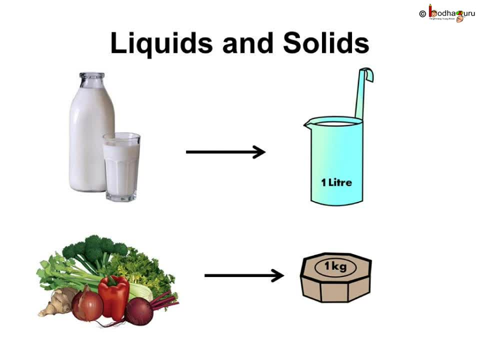 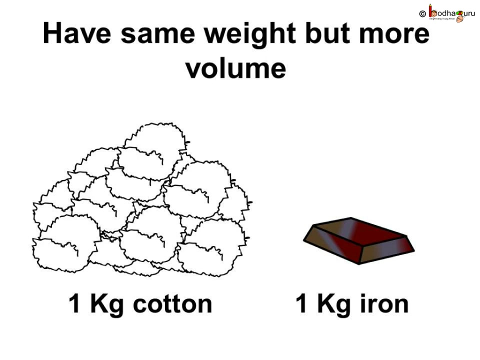 in kilograms or grams. Thus we buy these by measuring how heavy they are. We can measure volume of a liquid in liters and weight of a solid in kilograms. Normally when we increase the volume, the weight of the substance also increases, But volume of two different substances. 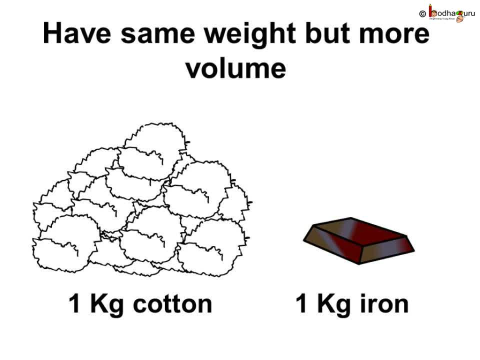 can be different, Like if we take a piece of iron that weighs one kilogram and a bunch of cotton that weighs one kilogram. we will find that their volume are different. Cotton occupies more space than iron. The amount of matter in a body is called its mass, As 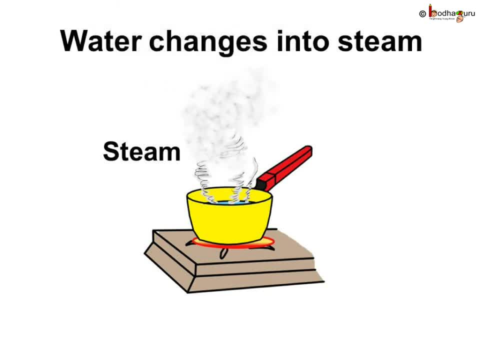 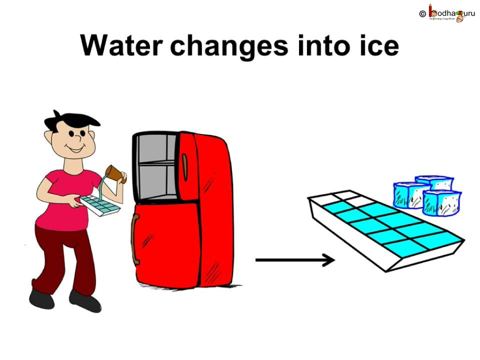 we saw Matters of solid liquid and gas can change their form when heated or cooled. Like water is a liquid, but when the water is heated till it boils, it changes into steam- that is gas. And if the water is cooled in a refrigerator it changes into ice that is solid. In this. 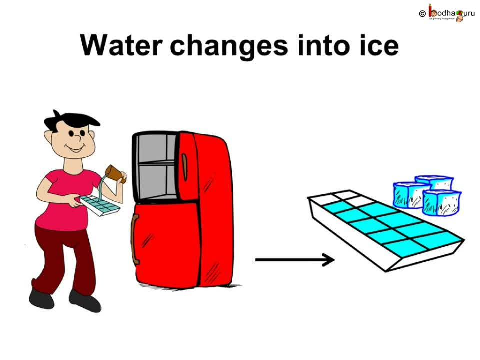 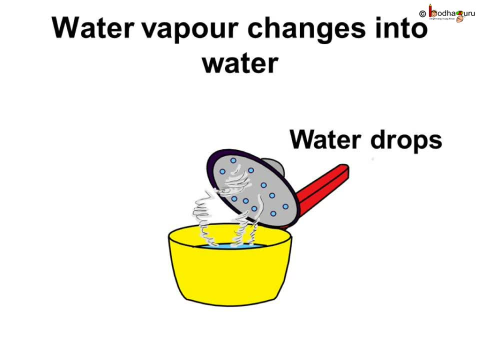 case, molecules of water remain the same, but the space between the molecules changes. This change can be reversed by reversing the conditions, like if we cool water vapor it turns into water, and if we heat the ice it becomes water again. 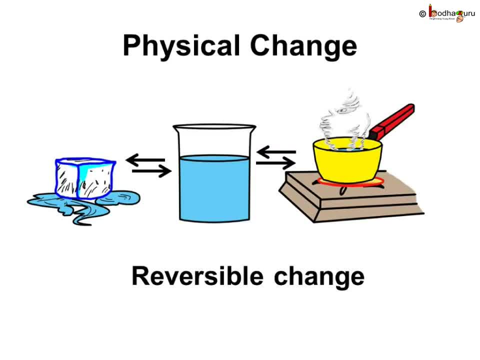 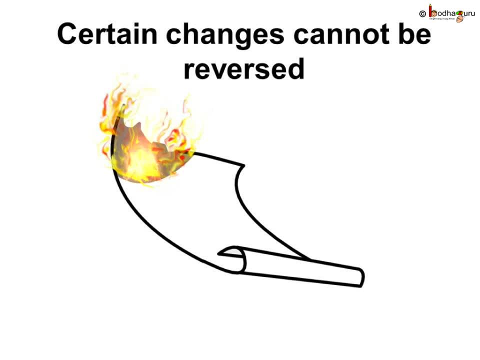 This kind of reversible change is called physical change. But what will happen if we burn a piece of paper and it changes into the ash? Is it possible to turn this ash into paper again? No, it is impossible. So there are some changes which are permanent and cannot be reversed. 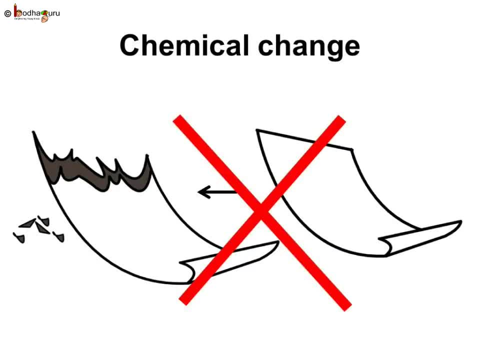 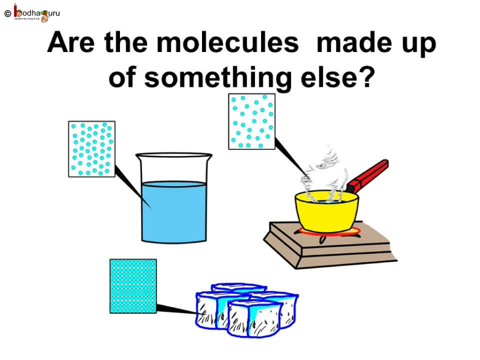 Such change, which cannot be reversed, is called physical change. This is called chemical change. So we know, when matter changes its state, the molecules of matter remain the same, only the space between the molecules changes. Now the question is: why are some changes reversible, that is, physical changes, and 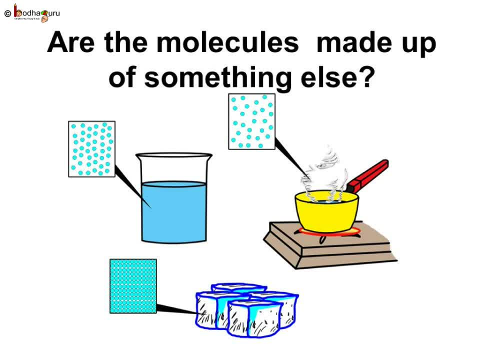 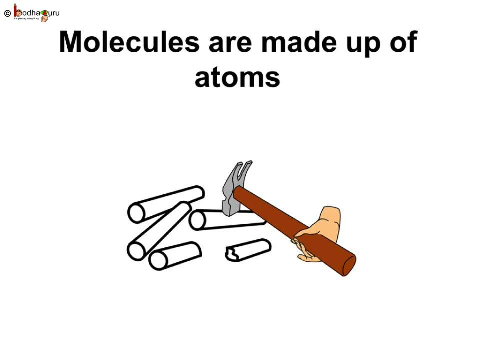 some are irreversible, that is, chemical changes. This is because the molecules are medium. The molecules are medium. The molecules are medium. They are made up of something else. Take a piece of chalk and break it into smaller and smaller pieces. Keep breaking the chalk until it can't be broken anymore. 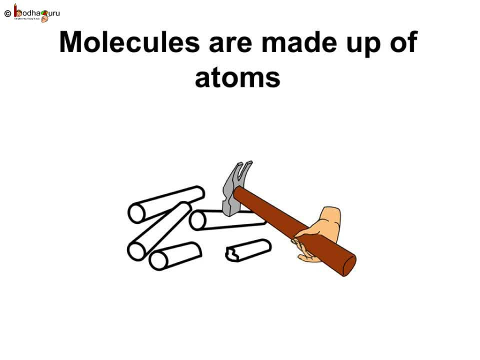 Now find out the single, smallest particle of chalk. Is it possible? No, because it is too small and cannot be seen even with the most powerful lens, with the most powerful microscope. These smallest particles are atoms. When atoms combine together, they form molecules And, as we know, all the matter is made up of molecules. So now we 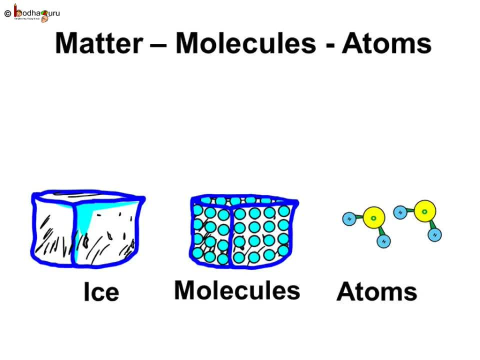 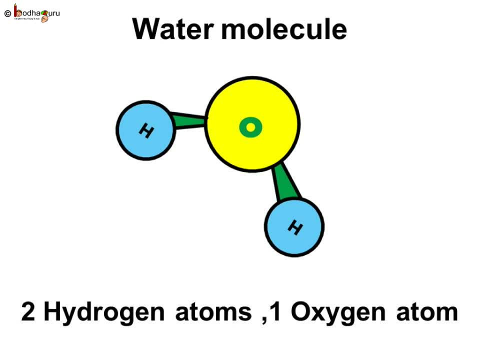 know, matter is made up by molecules and molecules are made up by atoms. There are some substances which are made up of molecules having the same kind of atoms, while some other substances whose molecules have different kind of atoms. It means if molecules break in the form of 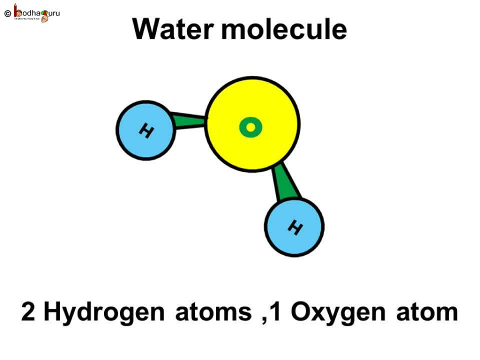 atoms. they will not be the same anymore. For example, in the water there are two atoms of hydrogen and one atom of oxygen, And hydrogen and oxygen are some names of atoms. When water changes into vapor or ice, the composition of molecule of water remains. 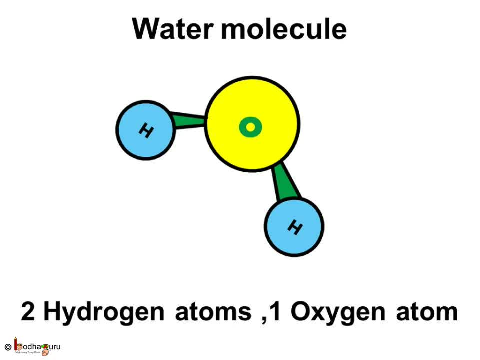 the same, That is, one molecule of water will continue to have two atoms of hydrogen and one atom of oxygen. Just the space between the molecule changes, And hence this change can be reversed back. ie, it's a physical change, But if we break the molecule of a, 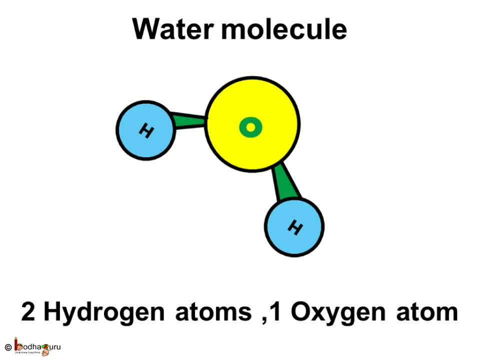 substance like the example of paper, turning it to ash. it is not the same substance any more. So in a chemical change the molecules break into atoms And atoms retain these molecules. Holler, Holler. So buy, So buy. 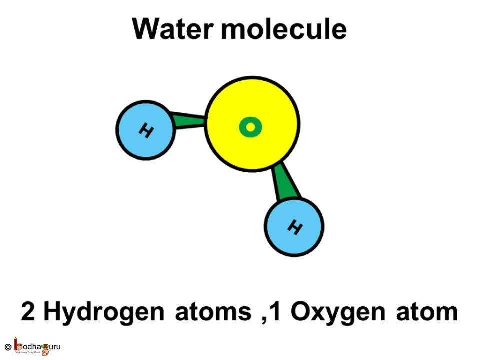 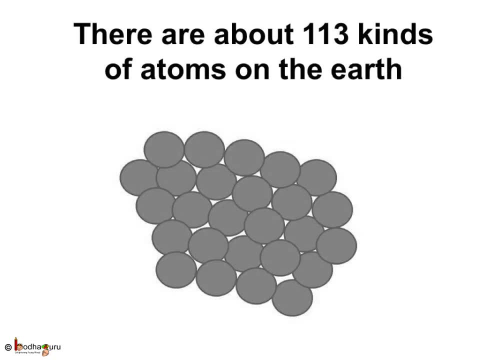 rearrange themselves to form new molecules, and hence this change is irreversible. You may think, if there are two types of atoms in a molecule of water, then there must be million kinds of atoms present in the universe, because there are so many things in the universe. 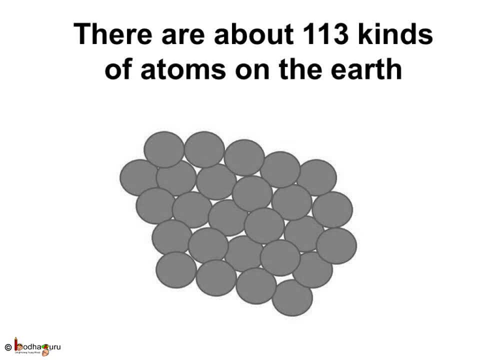 What you think is right, but it's not exactly like that. It will sound very strange, but there are about 113 kinds of atoms on the earth and by combining these atoms in different ways to form different molecules, we can make all the things in the universe. 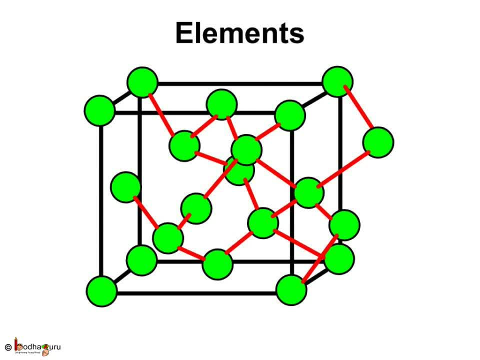 It is not necessary that all the molecules are made up by different kinds of atoms. It is not necessary that all the molecules are made up by different kinds of atoms. It is not necessary that all the molecules are made up by different kinds of atoms. 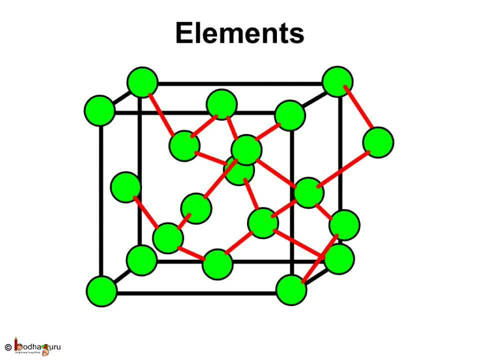 Some substances are made up of molecules having the same kind of atoms. They are called pure substances or elements. Oxygen, hydrogen, nitrogen, carbon sodium, iron, copper are some examples of elements. Their molecules have same type of atoms. Molecules which are made up of pure substances are called pure elements.